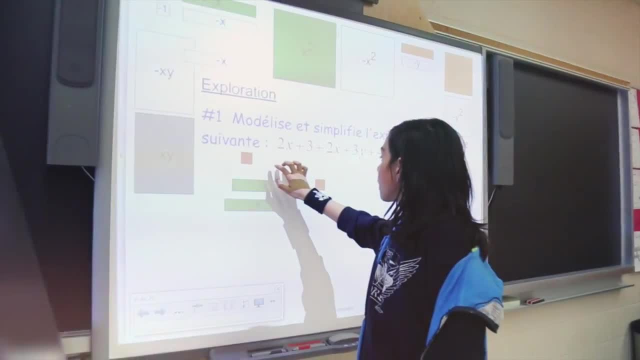 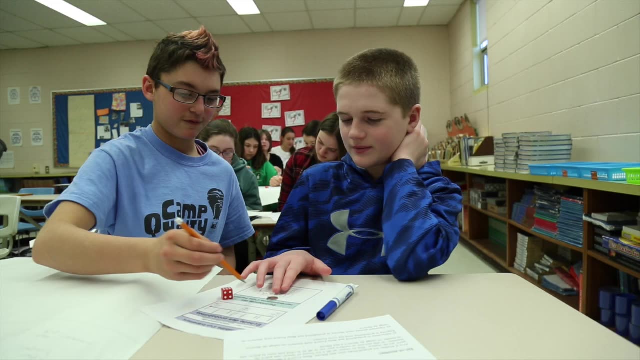 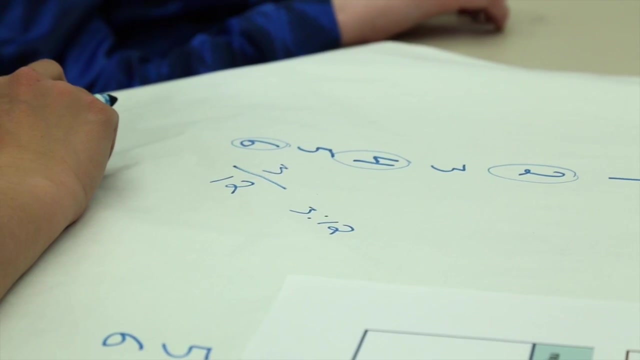 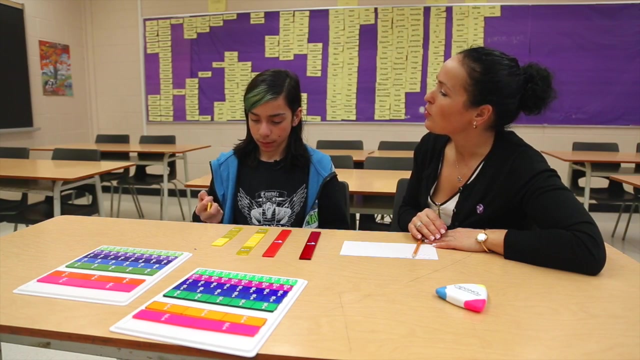 There are a number of problem solving strategies that students use in mathematics, but good problem solvers usually construct a representation of the problem to help them comprehend it. This can be particularly challenging for students with LDs, so it is important that educators help these students to understand the problem in a concrete way. 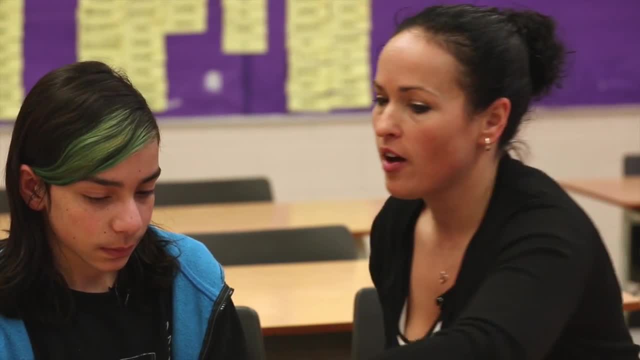 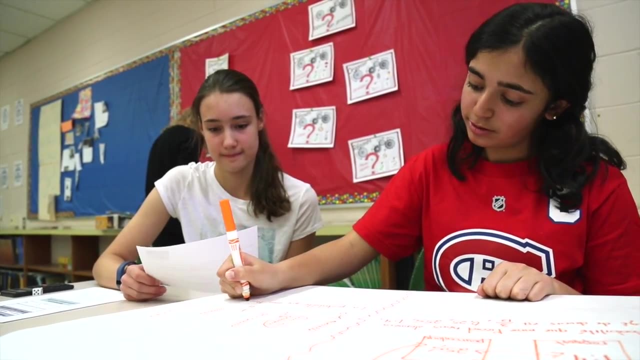 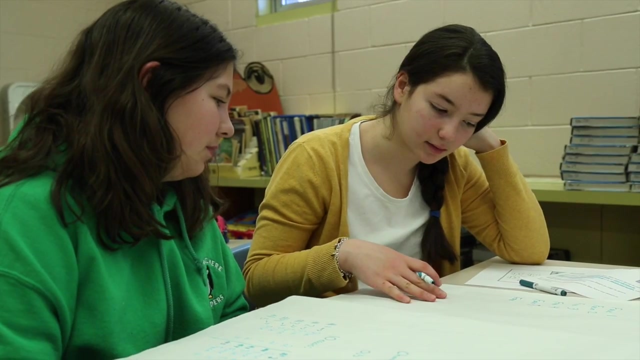 The use of manipulatives reduces the amount of information that students must hold in their working memory and increases the number of sensory inputs students use as they learn. This in turn improves the chances for them to remember the procedures required in problem solving. Consider the following math manipulatives to: 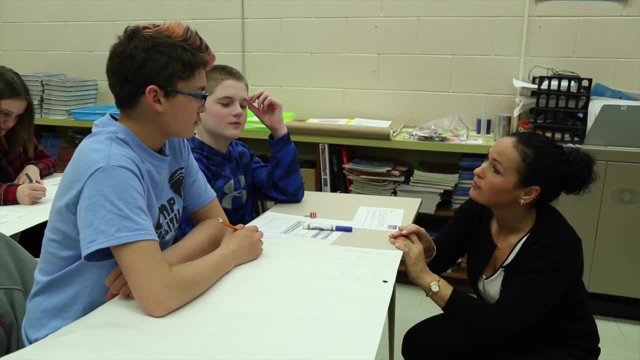 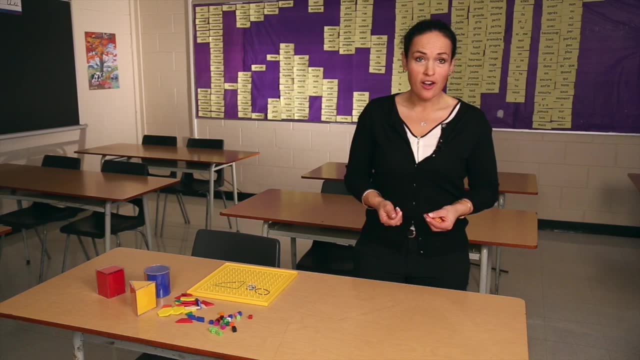 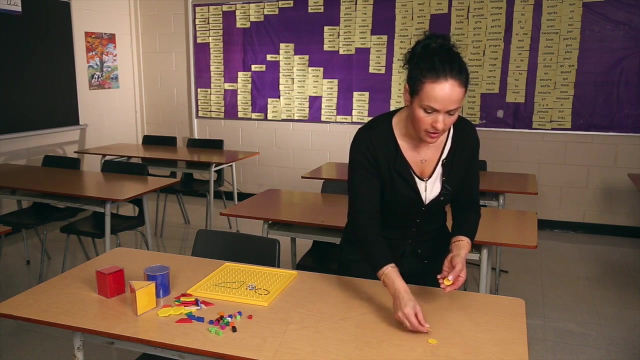 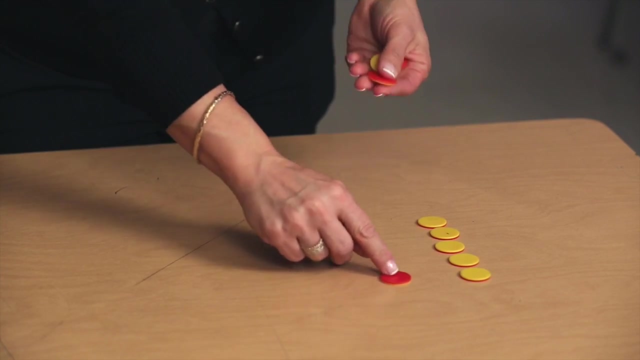 help your students gain a better understanding of a variety of mathematical concepts. When learning operations with integers, students can use counters of two different colors to represent expressions such as positive 5 plus negative 2.. They would use five counters of one color to represent the positive 5 and two counters of the other color to represent 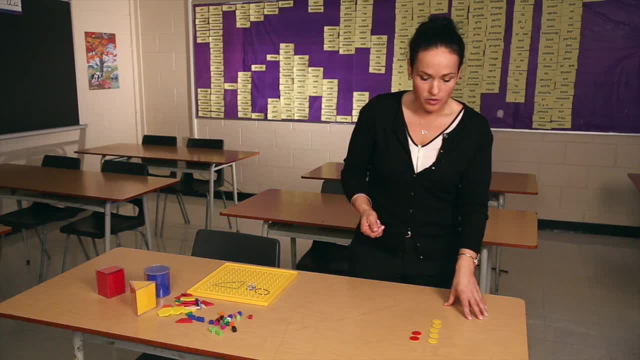 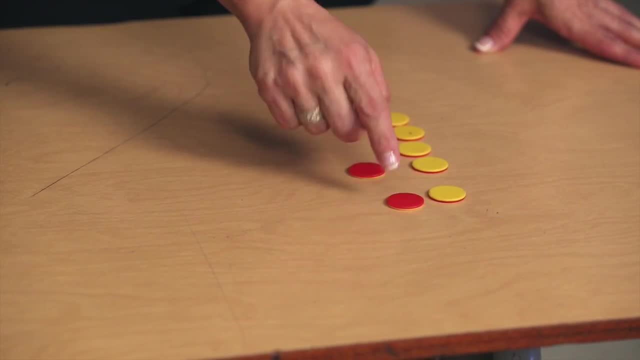 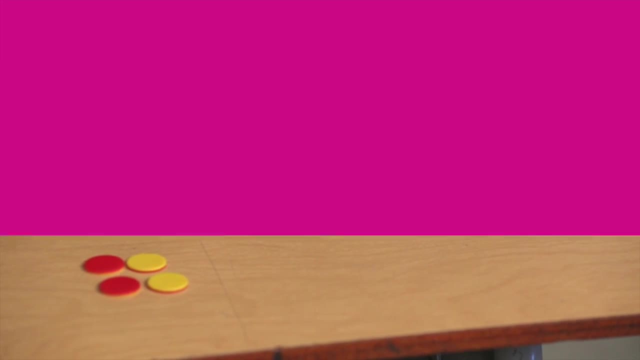 negative 2, as you see here. Then you can ask the student: how many is that all together? The student can conclude that positive 1 plus negative 1 equals 0, and so these counters can be eliminated here and here, And what you are left with is positive 3.. 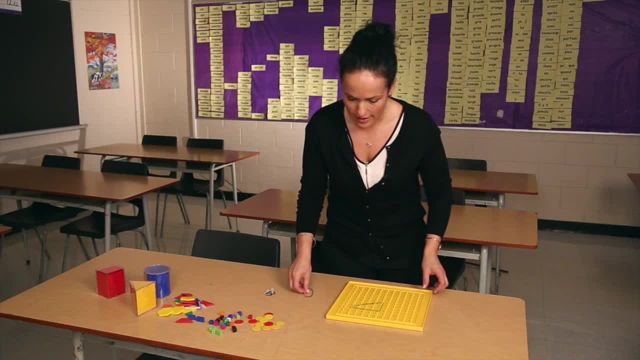 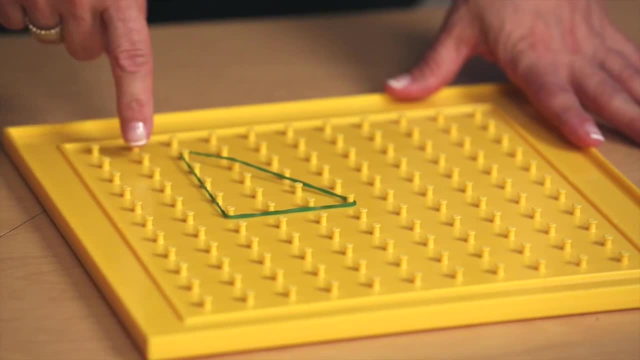 Working with a GeoBoard, you can ask the student to find the perimeter or the area of different shapes. We'll use the example of a triangle. If it's a discovery activity, students might compare the triangle to a rectangle, For a rectangle area is equal to the length times. 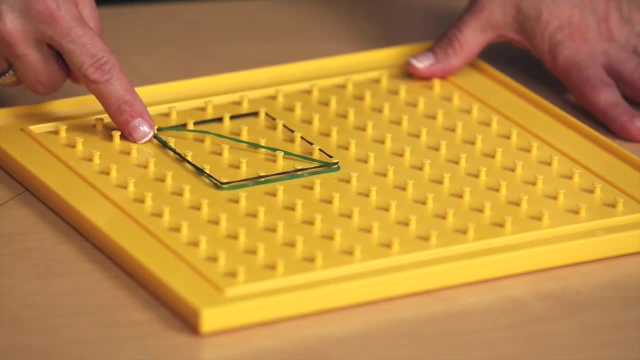 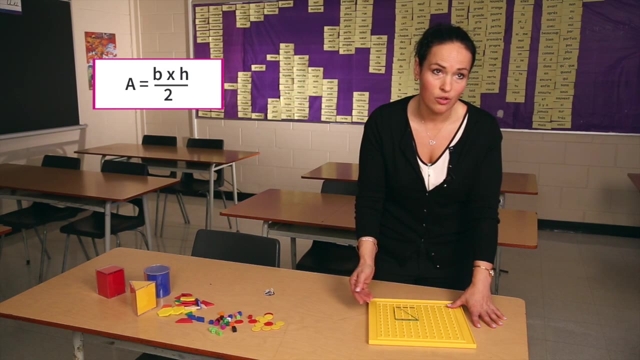 the width, In this case 3 times 4, which is equal to the length times the width. If we compare the two shapes, we see that the area of the triangle is half that of the rectangle. This helps students understand why we divide by 2 in the formula for area. 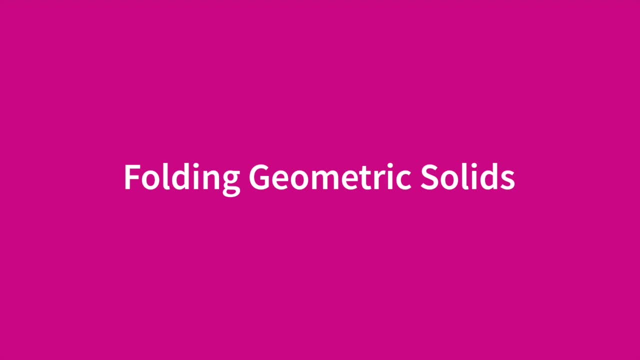 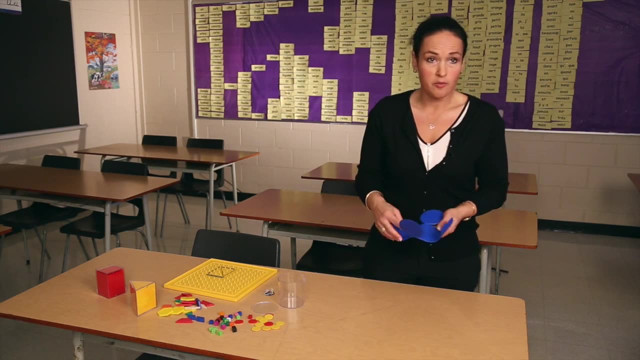 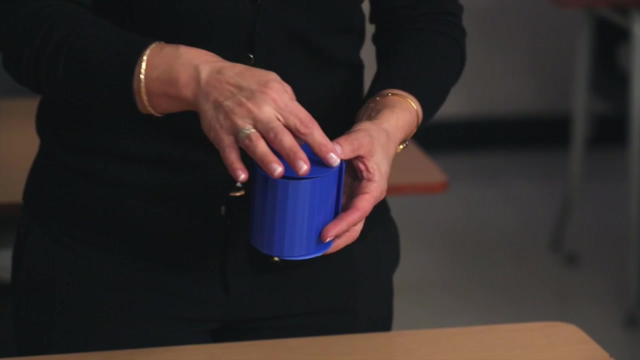 of a triangle. Folding geometric solids helps students understand the formulas for volume and surface area of three-dimensional shapes. For example, to find the surface area of a cylinder, students can use a ruler to measure the height as well as the diameter of the.